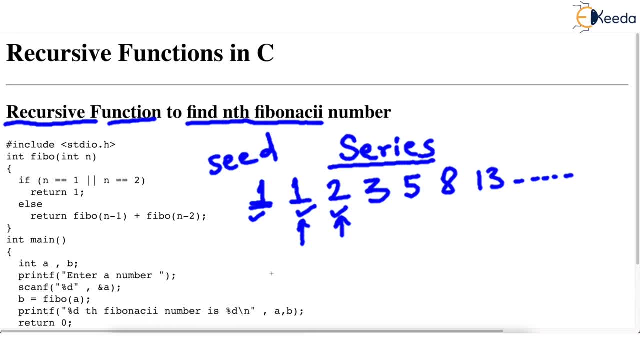 Like as an example, if I take first two numbers as 5 and 7, I am not wrong. Now these are the first two numbers- then the next number will be addition of previous two, and the next will be addition of 7 and 12, and next and so on. 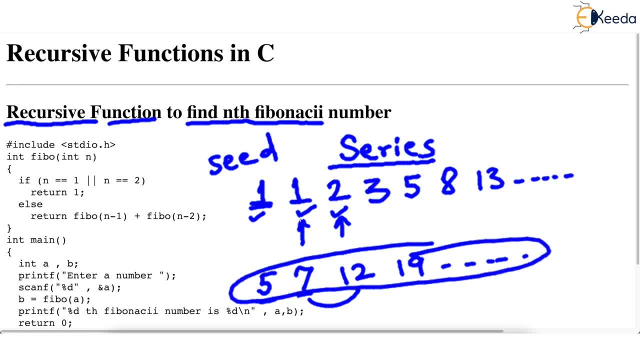 So this is my Fibonacci series, but typically we take the beginning as one one. There is no such rule that you have to take one one only as the beginning, but in our program we will take that as the first two numbers in the series. I hope that point is clear. Now, what really we want to do here? 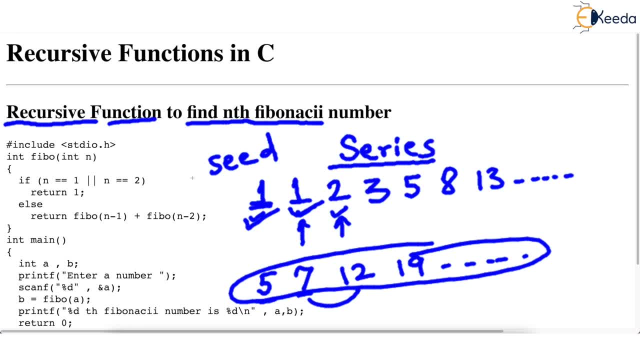 please try to understand is that we want to generate nth Fibonacci number. just observe this word: nth Fibonacci number. So here I have written a function, int Fibo. int n, n is the parameter. Let's say, I pass n as a in. Let's say, I pass N as n. n is a parameter. So if it is a parameter, I pass it by n. So it is a parameter and I have to pass n as n. So if it is a parameter, I have to pass n as n. 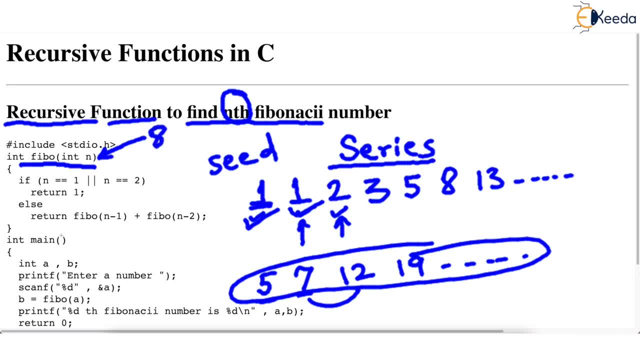 Let's say, I pass n as a integer. If it is a parameter, I pass n as n. So I have to pass n as a integer, n as 8. just check this. then i don't want to print all eight fibonacci numbers, rather first. 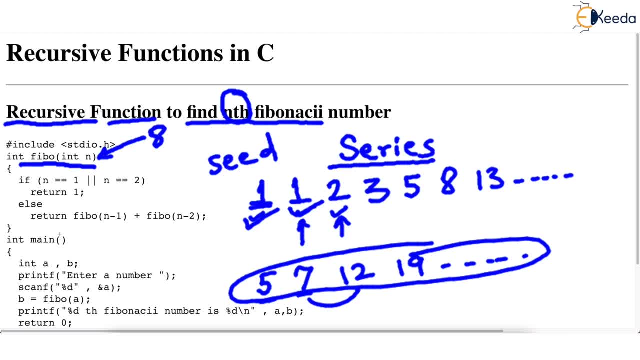 eight fibonacci numbers. i want only eight fibonacci number. just check this. that means, if you actually count this fibonacci numbers, this is first, second, three, four, five, six, seven and eighth one is going to be 21. so if i pass 8, 8 to this fibo function, then fibo function should. 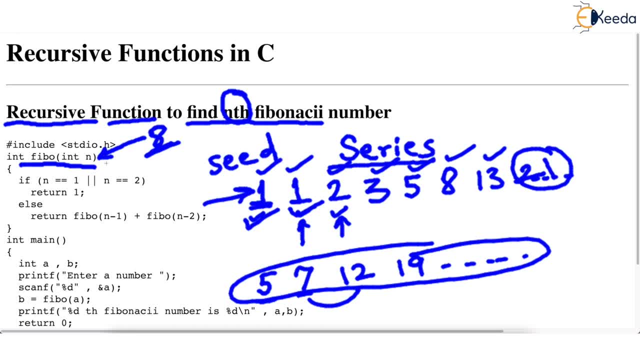 return only eighth fibonacci number, that is, 21, correct? that's the problem. as an example, suppose i pass, let's say, let's say i pass this n as as 6, then it should return sixth fibonacci number in the series, which is 1, 2, 3, 4. 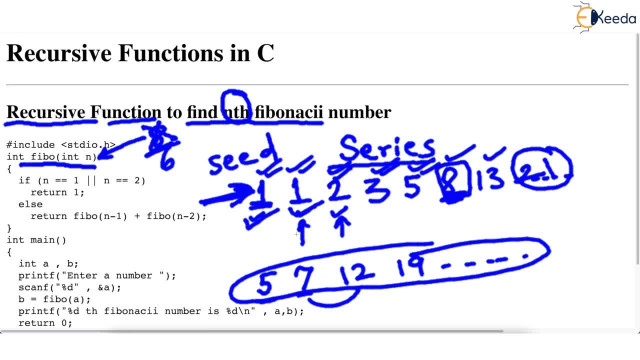 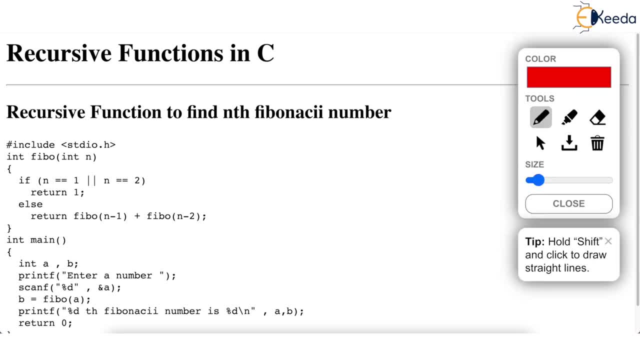 5, 6, 8, 8 is the answer. it should return okay. so i hope you got what is the problem, what exactly we want to do. now let's understand how to solve this recursively. check the recursive call here. for our reference, i will write the fibonacci series again over here: 1, 1, 2, 3. this was the 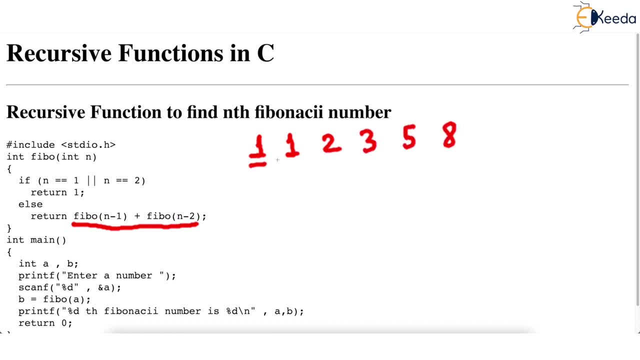 fibonacci series we were talking about with the first two terms as 1, 1. so i will write the fibonacci series again over here: 1, 1, 2, 3. this was the fibonacci series we were talking about, with the first two terms as 1, 1, 2, 3. this was the fibonacci series we. 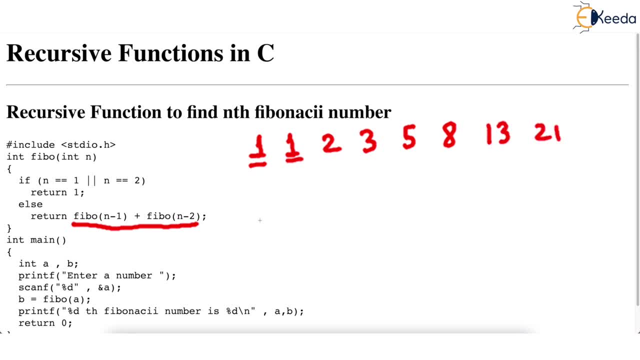 and this goes on. okay, now imagine that there somebody asks you again: what is fourth fibonacci number? so let's put up this question as fibo 4 in in the terms of function. so what is fourth fibonacci number? now, actually, you can observe that the fourth fibonacci number 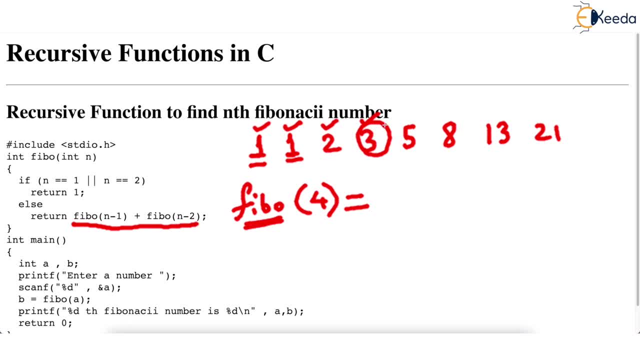 in the series is 3. okay, but we want to talk recursively, isn't it so? if you just answer fourth fibonacci number is 3, no, no, no, then you are not talking about recursion. you should say fourth fibonacci number is actually is actually third fibonacci number plus second fibonacci number. just check this and indeed it is. see, this is the arrow where i am. 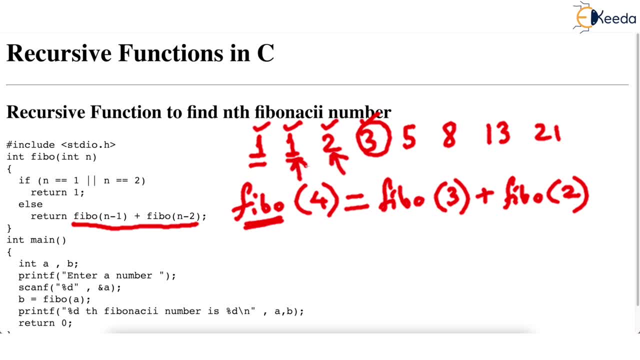 pointing is the third fibonacci and the arrow where i am pointing is the second fibonacci, isn't it? so this fourth fibonacci is given addition of previous two fibonacci numbers, but then obviously, what is third fibonacci? we don't know that, and what is second fibonacci? we don't even know that. but the third fibonacci is obviously addition of previous two, that is. 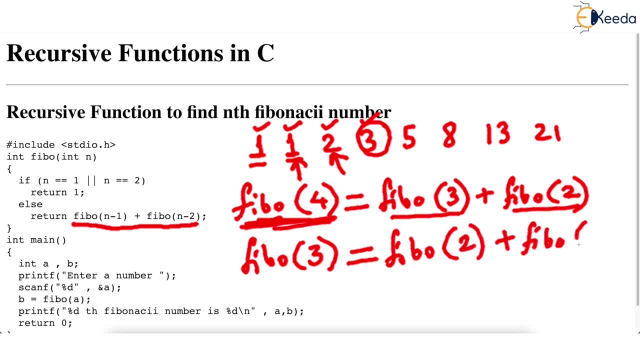 second fibonacci plus first fibonacci, isn't it? so you can see the recursion getting developed here. but then what is second fibonacci? coming back to the problem, what is second fibonacci? this, this problem. now, second fibonacci is one you can stop recursion because early in our explanation we said that first two fibonacci numbers are going to be. 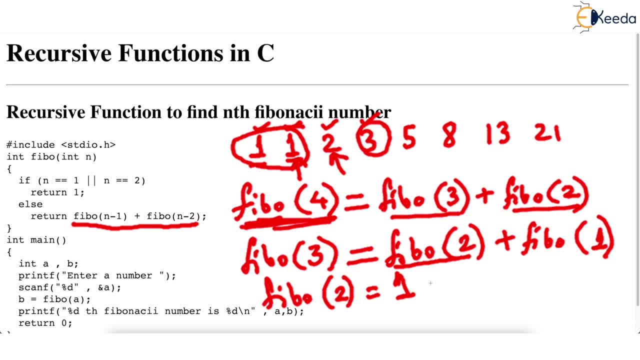 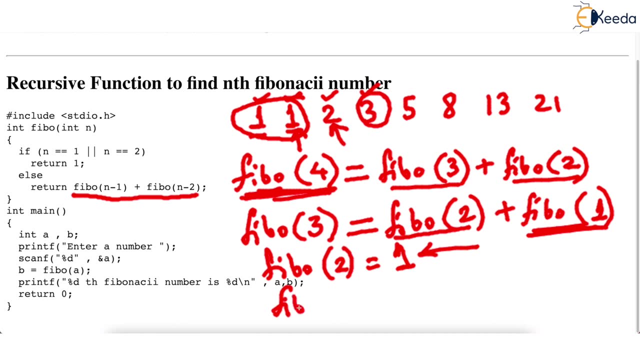 one one. that means, when we are asking what is the second fibonacci number, we won't say it is first fibonacci plus zeroth fibonacci. similarly, coming to the point what, what is the first fibonacci number? this one, fibo one, doesn't need any calculation. fibo one is one. i hope you got this, so can you. 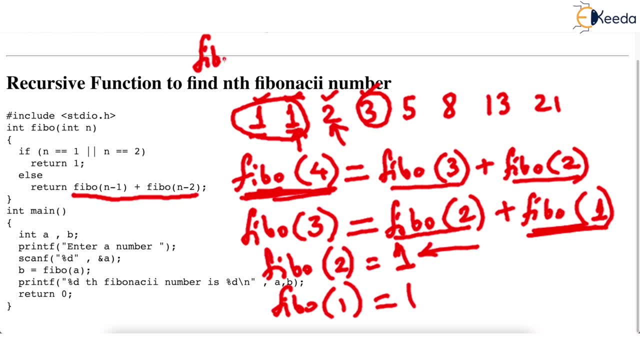 generalize it now. what is nth fibonacci number? nth fibonacci number? simple, this is n minus one to fibonacci, plus plus n minus second fibonacci. just check this. this is exactly what we have written on these lines. this is the recursive formula that we have got and nothing we have done. 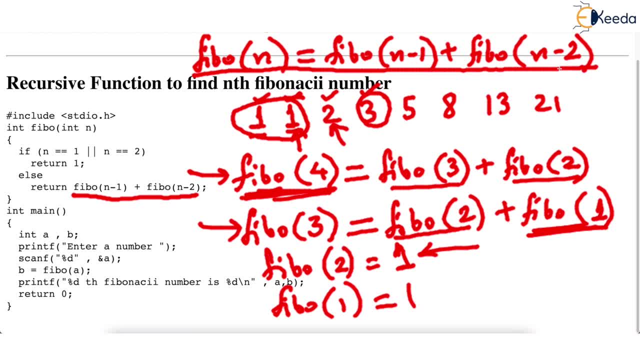 extraordinary. this was in the basic definition that if you want to generate nth fibonacci number, you must know just the previous two fibonacci numbers generated. but then you just observe: is this formula, is this recursive formula, applicable in all cases? no, in which cases is this not applicable? when n is one, that means you are asking which is the first. 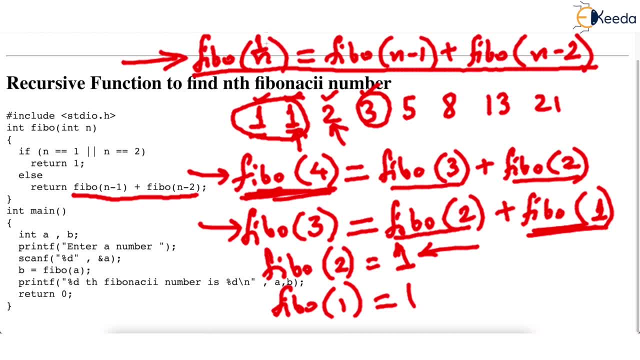 fibonacci you are asking, then it is rubbish when you are checking for the first fibonacci. if you say it is equal to zeroth. fibonacci plus minus one, fibonacci n minus one and n minus two are rubbish in that case. so this formula is not applicable when n is one. in fact, when n is one. 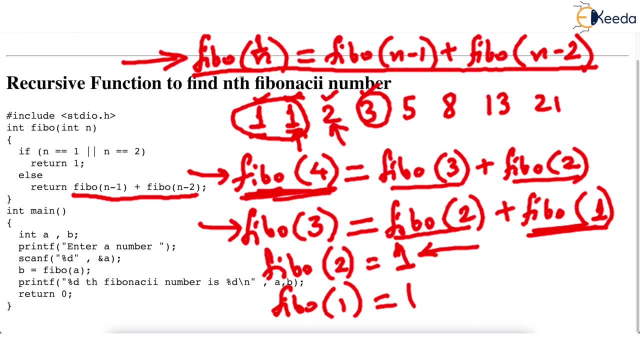 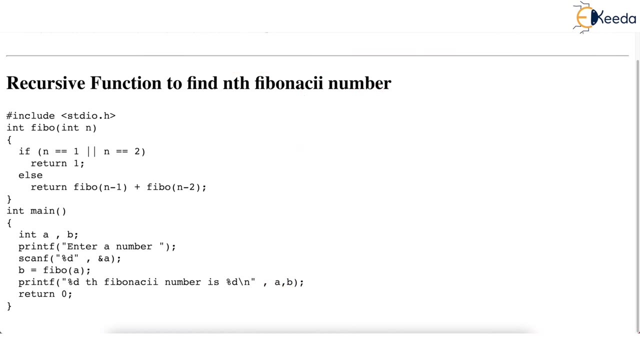 that is, you are asking for first fibonacci. you know that the answer is one and this formula is not applicable even when n is two. sorry for just i am overwriting a few things. when this n is two, then actually you want to know what is the second fibonacci, and second fibonacci is also one. hence we get, we get the recursive function. finally, 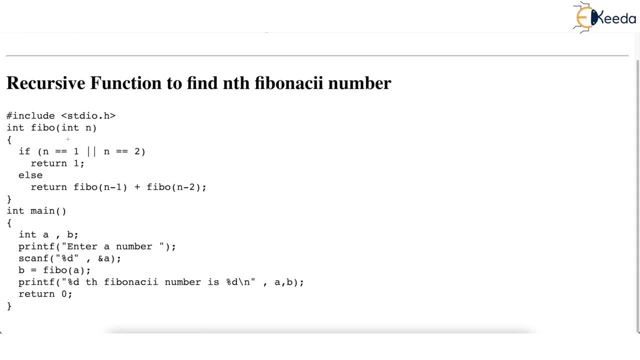 here. this is so easy. now, if you are asking for nth fibonacci, then first check the base case. if you are asking for first fibonacci, or check the or operator or second fibonacci, then don't do recursion but return one. otherwise return n minus one fibonacci plus n minus second fibonacci. this 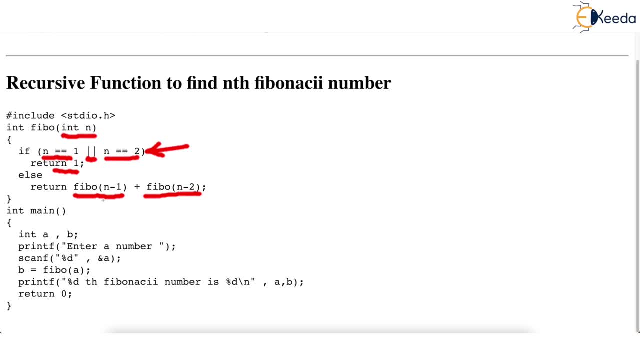 formalization. we just now wrote that nth fibonacci is equal to n minus one fibonacci plus n minus second fibonacci, main, is not at all extraordinary. we have two variables, a and b. ask the user to enter a. let's say i enter a as 8 and then i am calling the function saying b should become equal to fibo a.